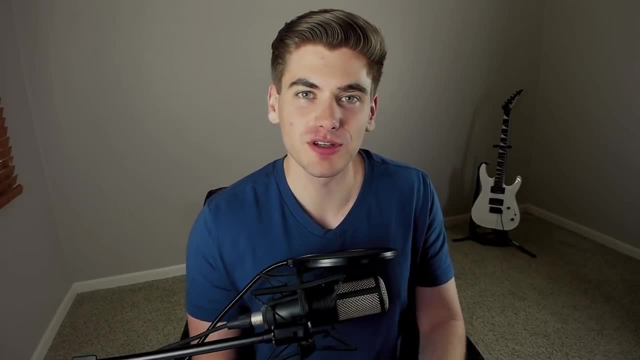 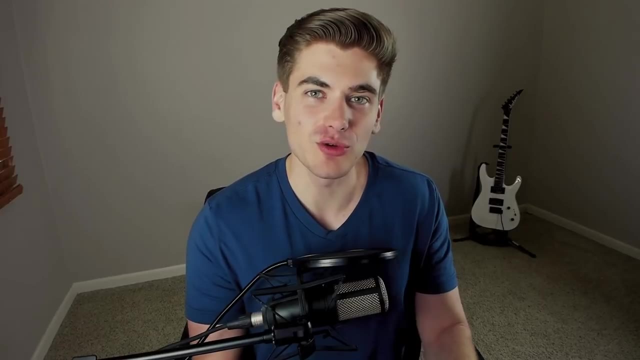 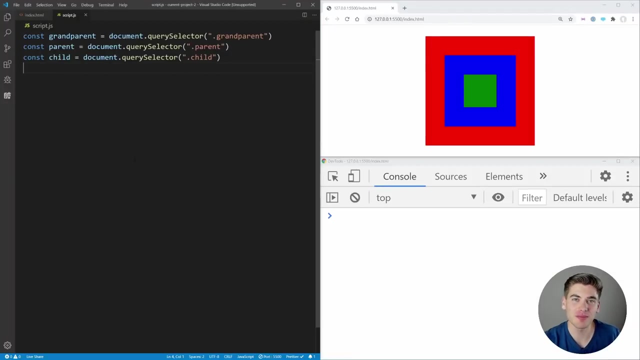 Whether you're a complete beginner just learning how to use event listeners, or if you've built multiple projects on your own using event listeners all the time, I can guarantee you there's something in this video you don't already know. Welcome back to Web Dev. Simplified My name. 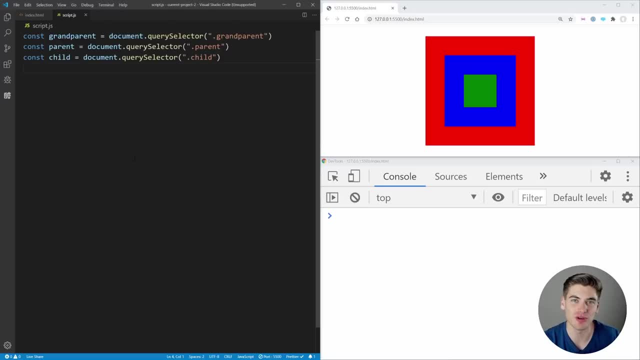 is Kyle, and my job is to simplify the web for you so you can start building your dream project sooner. So if that sounds interesting, make sure you subscribe to the channel for more videos just like this. Now, like I mentioned in the intro, we're going to be covering a ton of information. 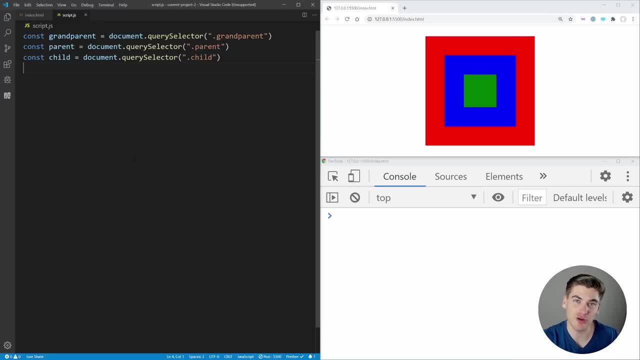 related to event listeners. We're going to start at the very basics of how you create an event listener and how they actually work. Then we're going to talk about capturing, bubbling and delegation and how all of that works, because it's incredibly important to understand and most 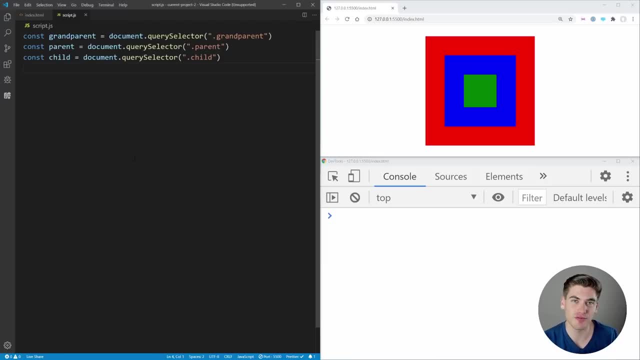 people really don't understand it well enough. And then, finally, we're going to talk about a few minor tidbits here and there of bonuses that come with event listeners. So this video is going to be jam-packed full of information, so make sure you stick around till the end to get all of the 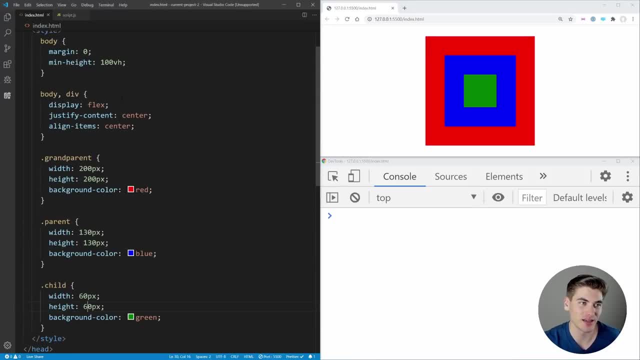 information you need Now to get started. I have a really simple indexhtml file where we have a grandparent, inside that we have a parent and inside that we have a child. And you can see, on this right-hand side we have this red grandparent, blue parent and then green child. And what we're going to do? 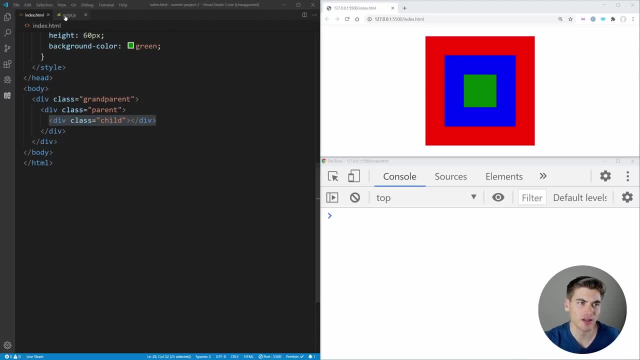 is set up event listeners for when we click on these elements. So the very first thing I want to do is set up a click event listener on the grandparent. In order to do that, all we need to do is take the grandparent element, so just type in grandparent and we put a period And as 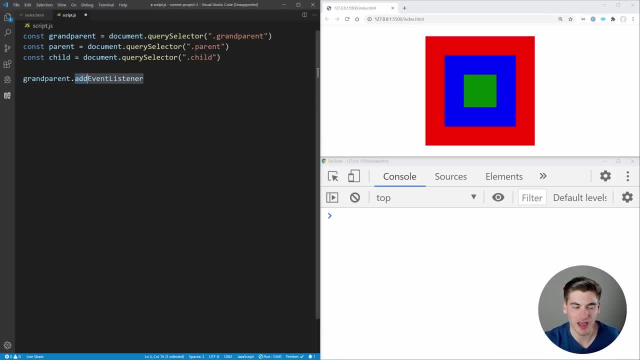 you can see, the very first thing on this list is called add event listener. So we're going to just type in add event listener and this is going to take two to three parameters. For now we're just going to start with the two parameter version because that's the most common. The first 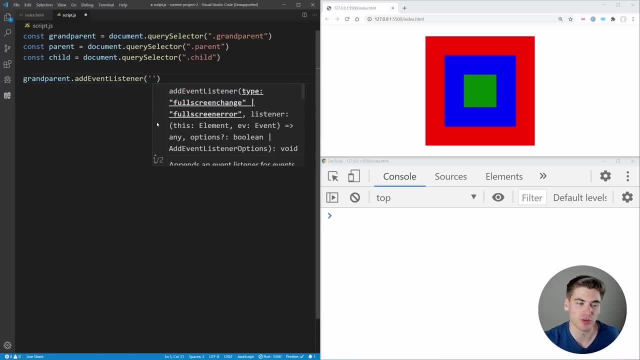 parameter you put in here is going to be the type of event that you want to listen for. In our case, we're listening for a click event. There are tons and tons of events you can listen for and if you want to know what they're called, just google. you know, mouse down event or mouse over. 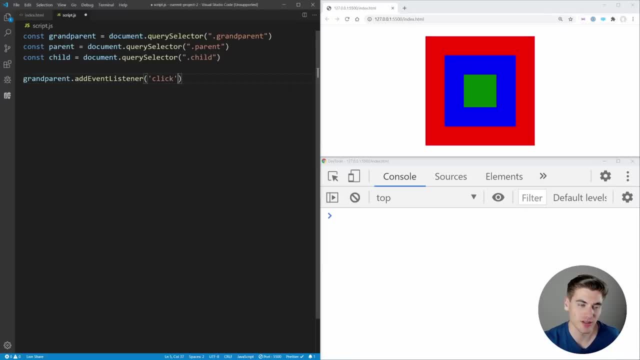 event and it'll give you the exact name that you're looking for if you don't already know it. The next thing we need to pass here is a callback, and this callback is just a that runs every single time that we do, whatever the event is in our case, click And this takes. 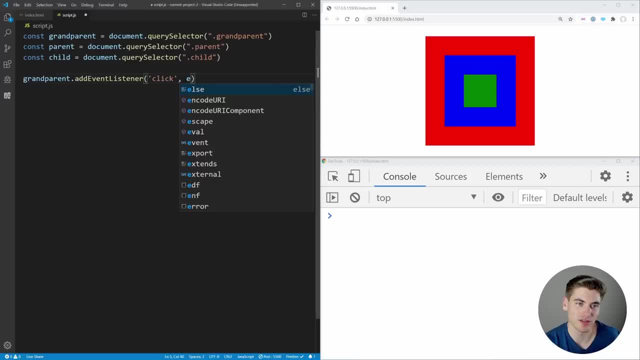 a single parameter, which is the event object. Generally, you'll see this called e. We're just going to use an arrow function for our use case. If you don't already know arrow functions, make sure to check out my video linked in the cards and description. It covers arrow functions in depth. 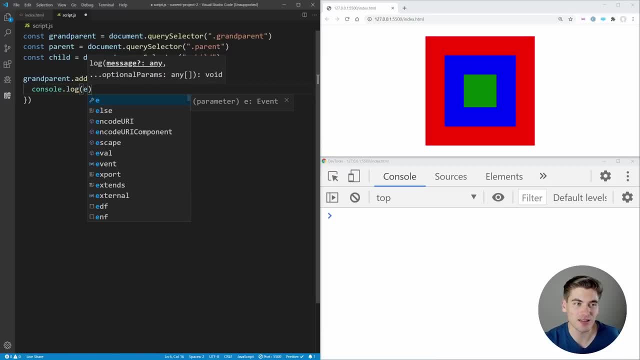 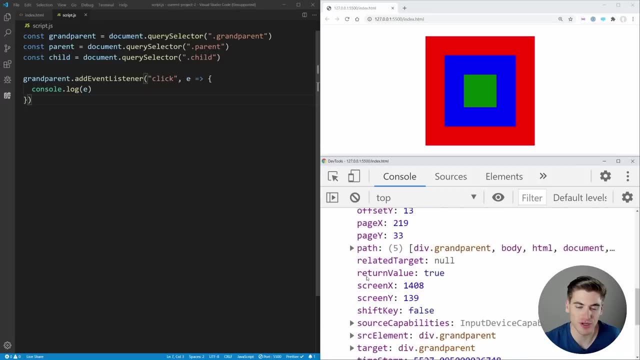 So now let's just come in here and do a console log of e to see exactly what this e is. So now, if we just come over here, click on the grandparent, you're going to notice we get this massive event down here with tons of information inside of it. 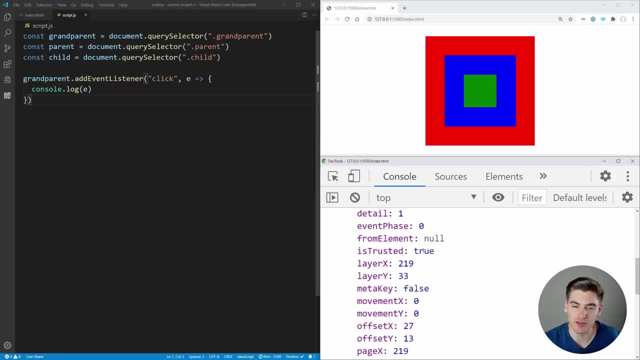 A lot of this information deals with where your mouse is on the screen. It deals with where you're holding down, like the control key, for example. There's a bunch of information inside of here, but probably the most important information that you're going to care about is this thing. 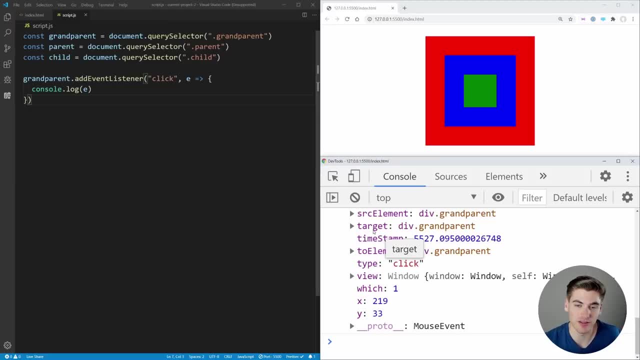 called target right here. Target is essentially the thing that you clicked on, in our case the grandparent. So that is the target, and target is just an element, so it has all the normal element-related information inside of it. But generally when you're dealing with click, 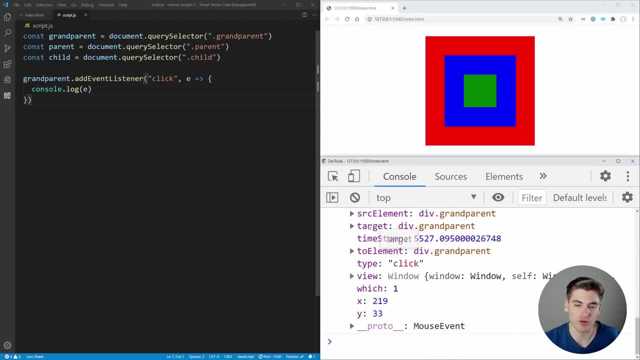 event listeners or any event listener target is usually the most important thing that you want to mess with inside of the event listener, because it is the thing that you're going to care about. So in our case, that would be this grandparent. So if we just consolelog etarget and I click. 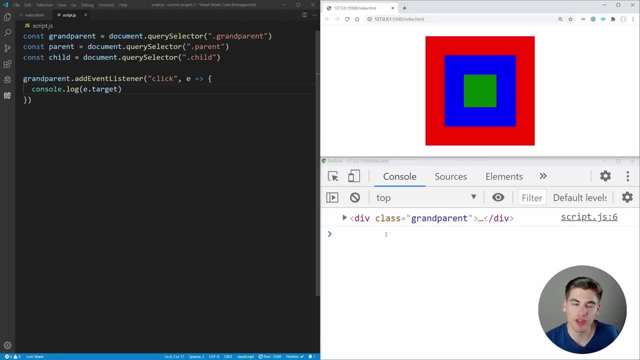 on this again. you're going to see it prints out that grandparent element. Now, one thing that's also interesting about event listeners is we'll just change this to print out grandparent1.. What we can do is add multiple event listeners. So if I just copy this, paste it down here and put. 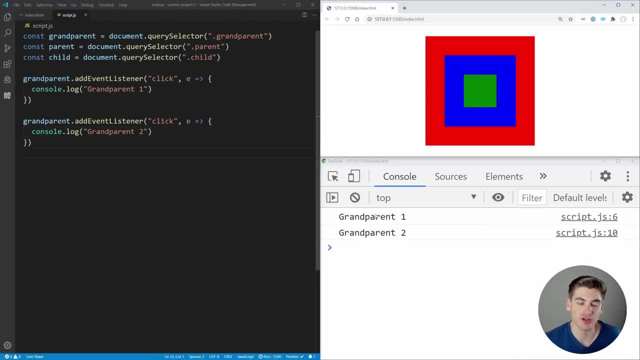 grandparent2 inside of it and I click save. when we click on this, you're going to notice it's going to run both of the event listeners in the order that we defined them. So grandparent1, goes first, because that's the first one we defined, and then grandparent2 comes second. 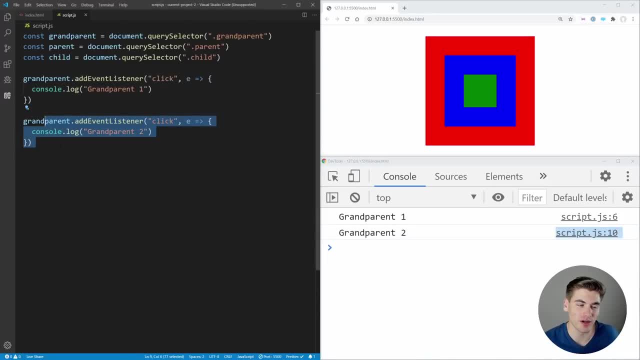 because that's the second one that we defined. That's the default behavior of event listeners And this, right here, is what most people understand when it comes to event listeners: They know how to put the type in, they know how to create a callback function and they know that they run in the order. 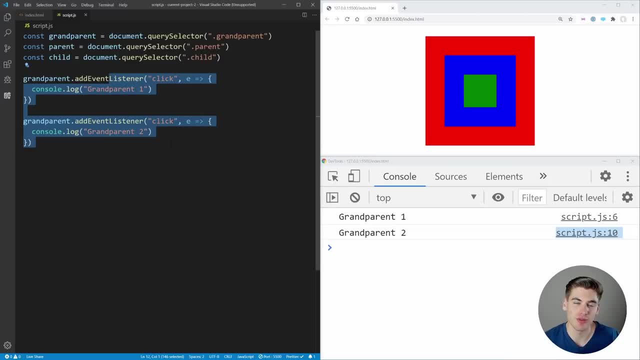 that you define them, and it's about where most people's knowledge stops. So in the rest of this video we're going to go beyond just this basic information and talk about everything else that there is to know about event listeners Like, for example- you'll notice when I click on this child- 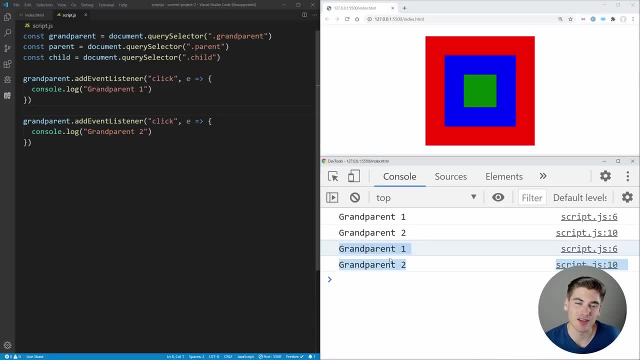 it still prints out the grandparent information. Why exactly is that? Well, to figure out, let's first set up event listeners for our parent and our child. So let's just come in here, we're going to copy this grandparent1, paste it down, and in here we're just going to say parent and this: 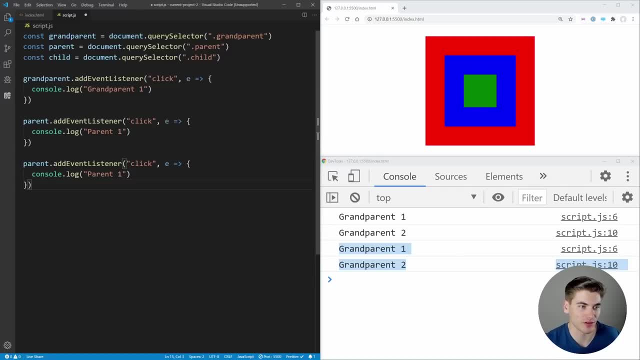 will just say parent, and then we're going to do the exact same thing for child. So here we'll say child and child. So now if we click grandparent, it'll print grandparent. When we click on the parent, you're going to notice it prints out grandparent1,, grandparent2,, grandparent3,, grandparent4,. 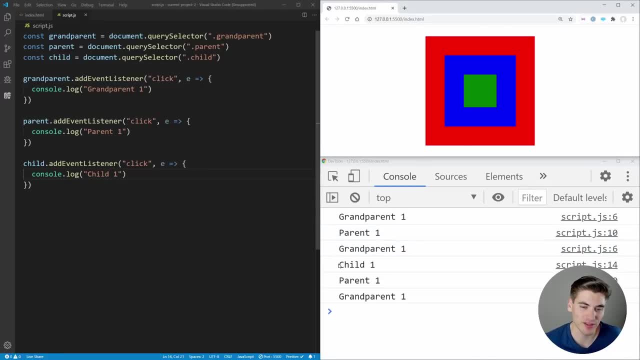 parent1, and then grandparent1,. and now when we click the child, it's going to print child1,, parent1, and then grandparent1.. So if you're paying attention, essentially what's happening is that we're clicking on this element, but behind this green child is also our blue parent. 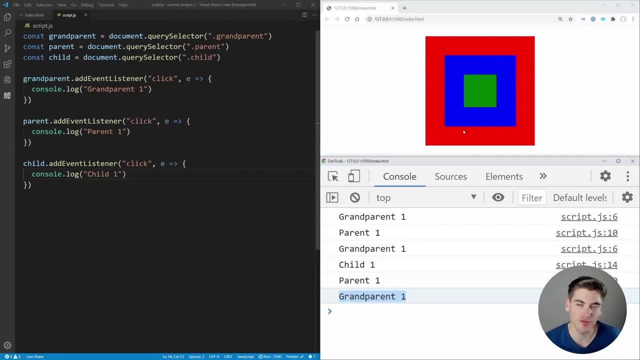 and behind our blue parent is our red- you know grandparent here, And even further behind that is our actual document itself, which we could set up an event listener for, For example, documentaddEventListener. click and we're just going to come in here. 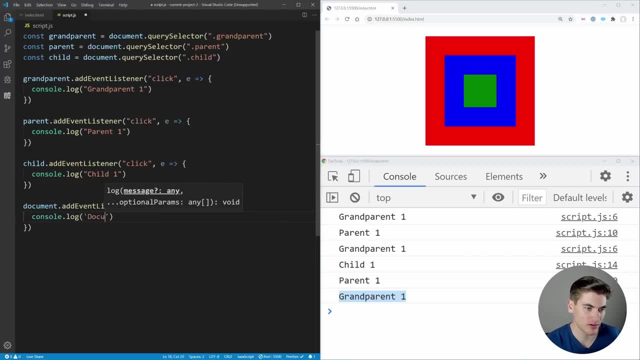 and we're going to consolelog document1.. So now if we click the document, it prints out document. we click here, it prints out child, parent, grandparent, and then document. And that's because it's working its way from the closest element, in our case this child, all the way to. 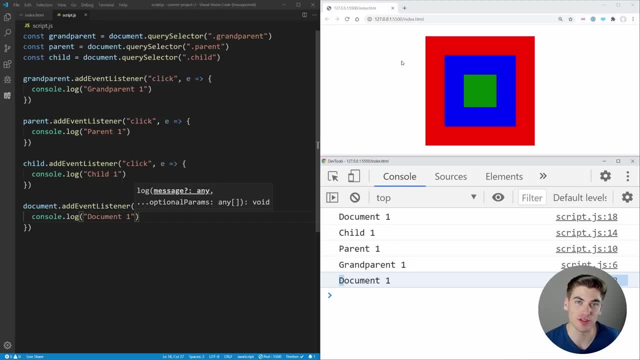 the furthest away element, which is our document And it's running click event listeners for all of them, because we technically clicked on all of them, since the child is inside the parent and the parent is inside of the grandparent and the grandparent is inside of the whole document. 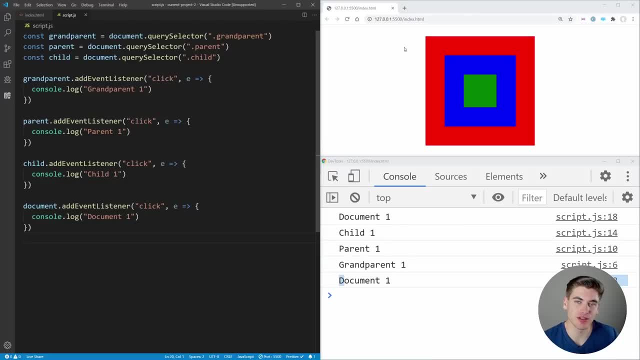 itself. This process of going from the closest element to the furthest away element is something called bubbling. You also may hear it called event bubbling, and this is one half of how events work inside of JavaScript. The other half of how. 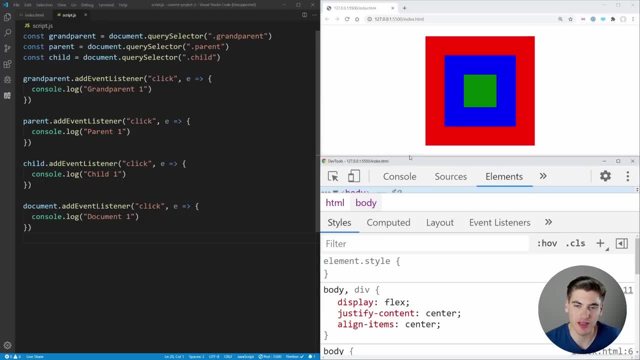 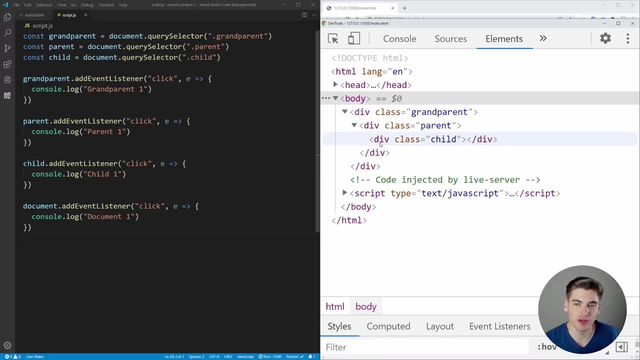 they work is called capturing. So if I just go to this elements tab here, I'm going to expand this up so we can really see what we're working with, get it as large as I can and open up the grandparent, parent and the child So you're going to see at our very first when we click. 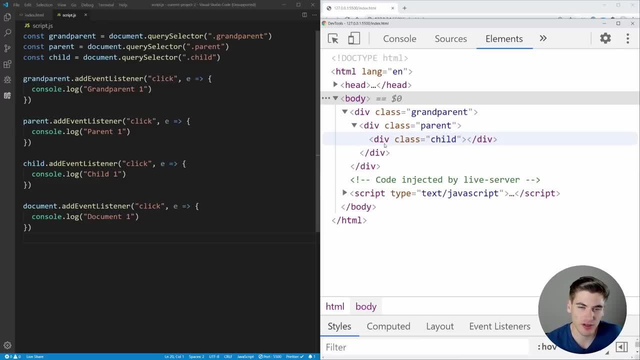 on our page we click inside the child right. So our click is going to start at the child here. it's going to go down to the parent, go down to the grandparent and then all the way down to the document as its final step. It's kind of working out of its 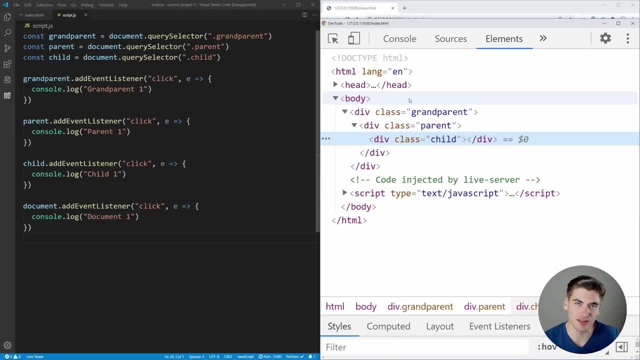 hierarchy because we clicked on all of them. Well, that is, like I said, the bubbling phase. There's a second phase called the capturing phase, and this actually happens first. The way the capture works is it works for the thing furthest away and moves up. so it'll start with the 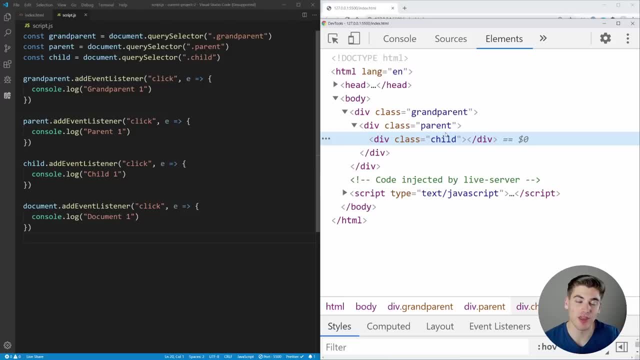 document, then the grandparent, then the parent, then the child. then we swap over to the bubble phase, where we go from child to parent, to grandparent, back to document. The way to remember this that I like to think about it is when you bubble. generally bubbles move up. 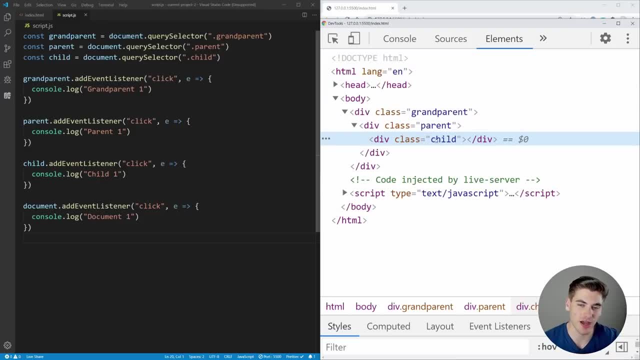 because they're light. so you bubble up the tree. so you start down here, at the lowest, most minute element, and you bubble upwards out of the tree. That's how I like to remember capturing versus bubbling. Like I said, capture starts on the outside, moves in and then bubbling. 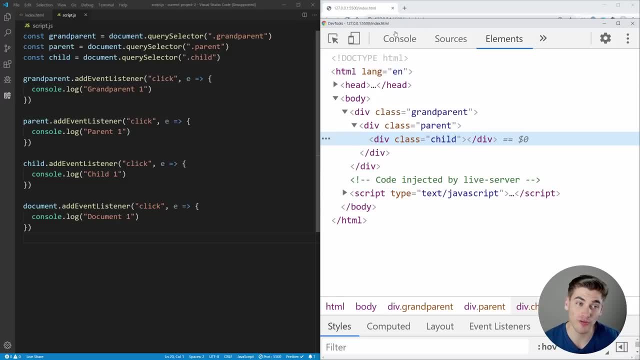 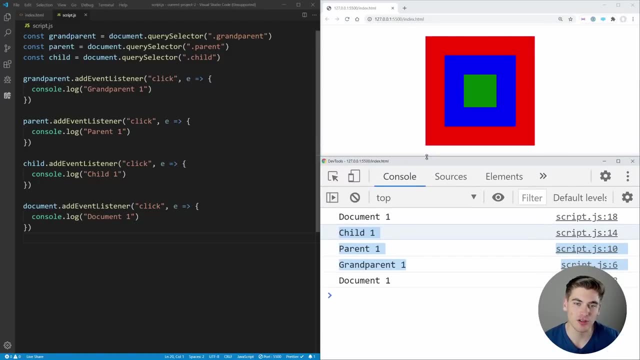 happens second and goes from the inside out. But right now all of our events are bubble events because, as you notice, we print child, then parent, then grandparent, then document, in that order, because they're all bubbling. So how exactly do we do a capture? That is where this third parameter 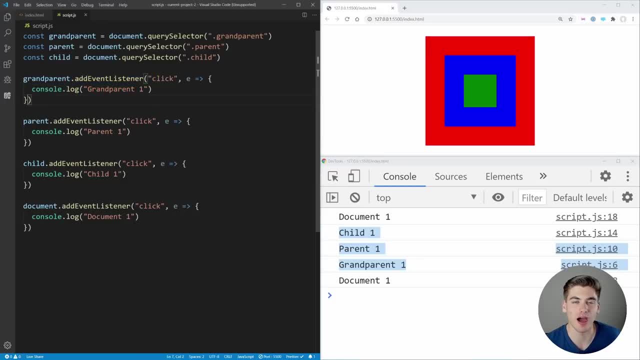 to the add event listener comes in. So we're going to go to the add event listener and we're going into play. We can pass in here an option, and these options is just an object where we pass in different parameters to it, So we could pass capture and set it to true By default. this is. 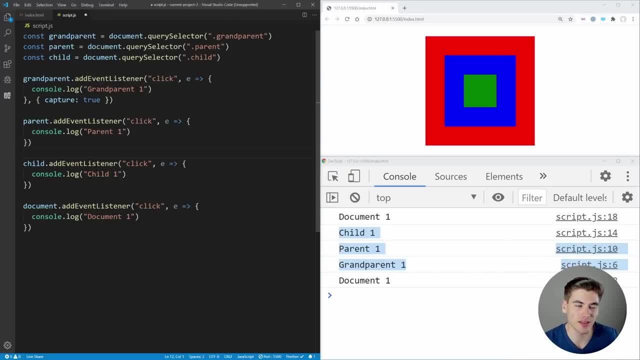 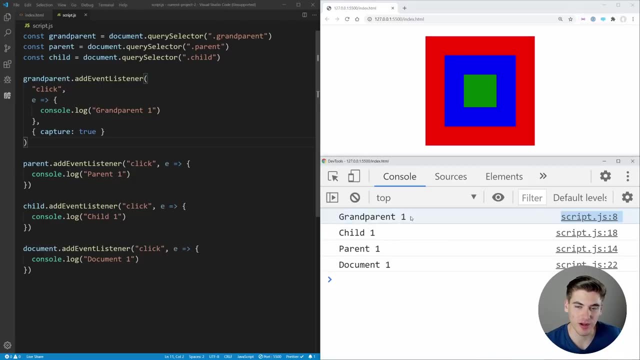 set to false, but if we set it to true, we're saying we want this event to be a capture event. So now, if I save this and I click on the child, you're going to notice something interesting: It prints grandparent one, then child one, then parent one, then document one. and that's because our 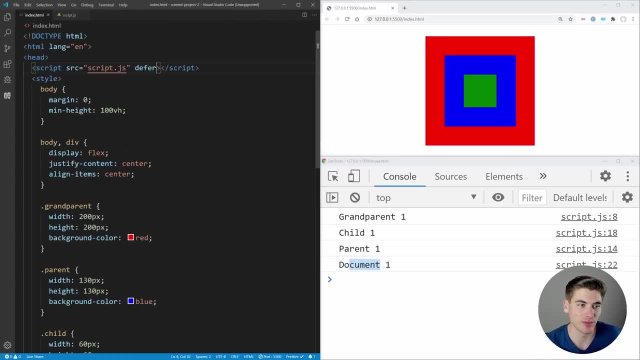 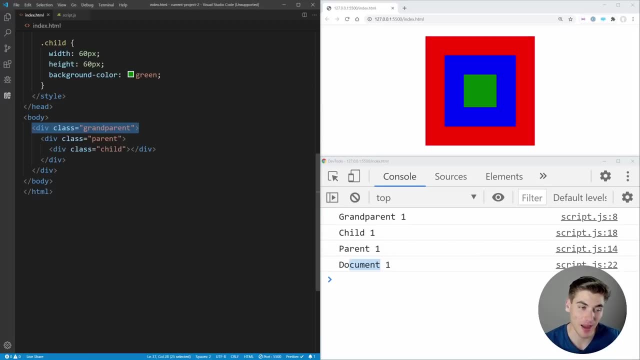 grandparent is in the capture phase. So if we just go to our HTML here real quick, what's happening is we start with the capture, which means we start at our document, then we move to our grandparent, which we set up a capture event on, so it prints out here: 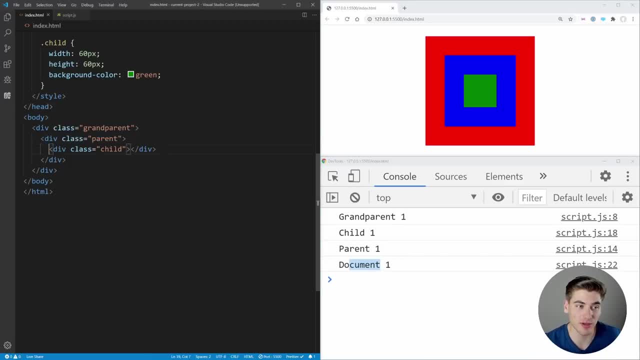 Then we do the capture for our parent. There is no capture event, so we skip it. Do the capture for our child. Again, there is no capture for our child, so we skip it. And then we do the bubble. So we bubble our child where it prints out child one. Do the bubble for. 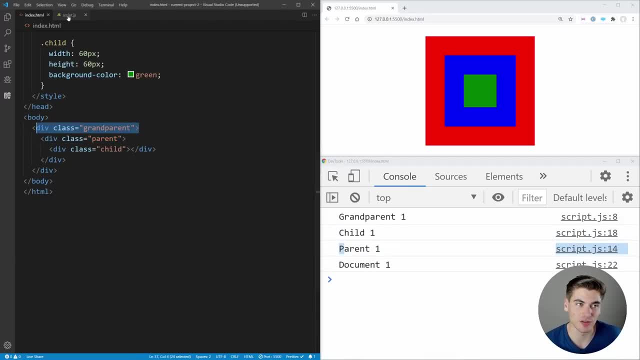 our parent, where it prints out parent. one Bubble for our grandparent and since we swapped this to a capture event, there is no bubble phase, so it skips it. And then we do the bubble for our document, which finally finishes the capture. And then we do the bubble for our child, where it 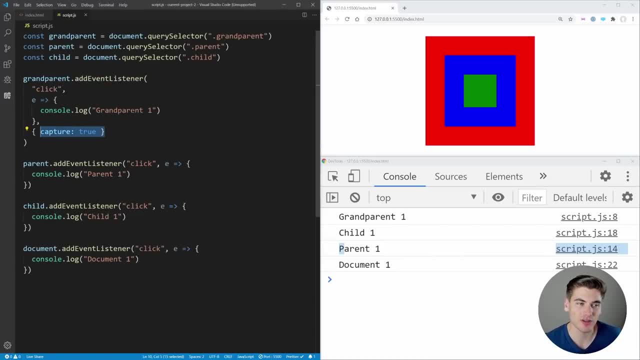 all off. So this is how the capturing and bubbling system works, And to really see in depth how it works, what I want to do is just copy all of these events so we can have grandparent capture, and then we're going to have grandparent bubble, which is just the default. So I'm going to 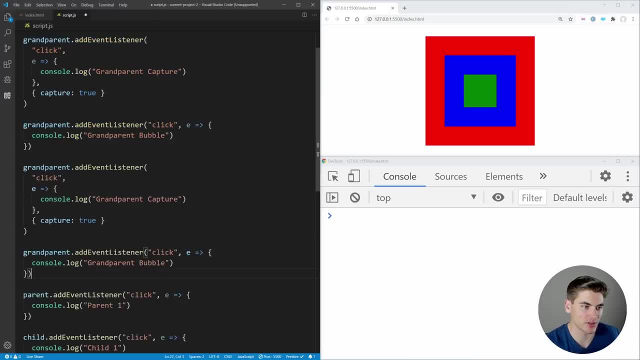 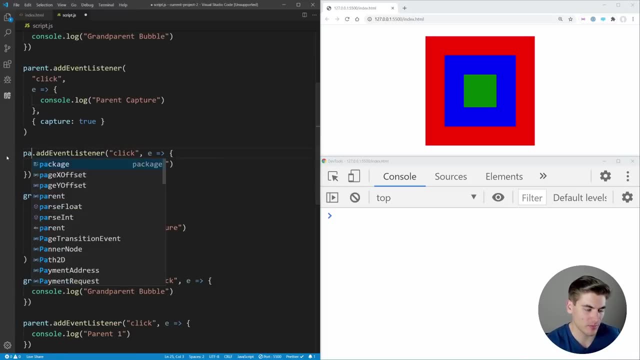 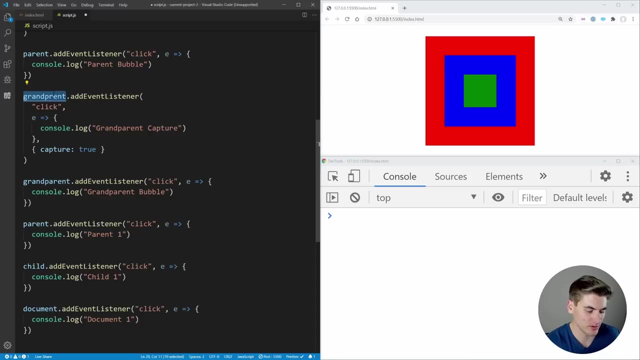 remove that and I'm just going to copy this down a couple times So we have all of them. So we got the parent. This is going to be parent capture, Parent here, Parent bubble. Then we're going to have our child And our child capture. Then we're going to do the. 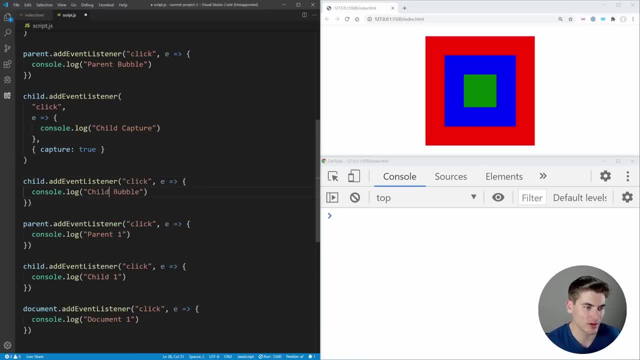 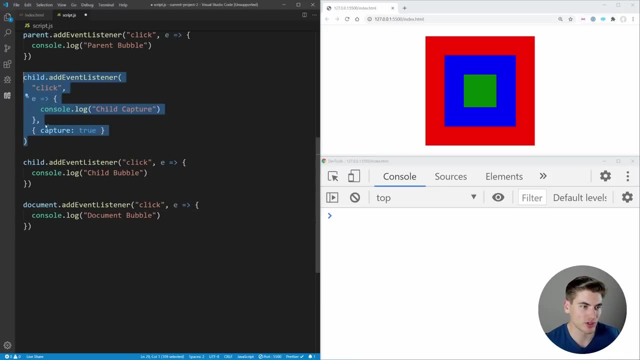 bubble for our child right here, So child bubble. And then we can even finish this off by doing the document as well. So we got document bubble and we each copy this. We can get the document capture as our final one, The document here. Document capture. 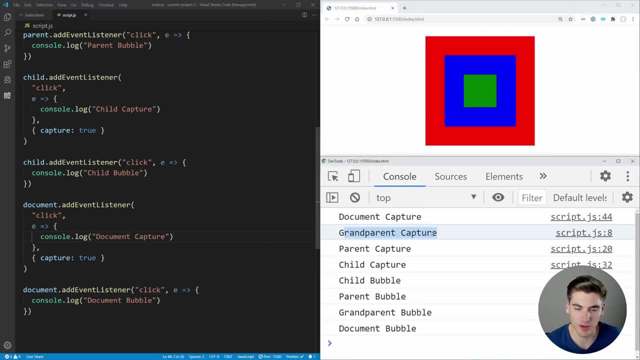 Now if I click on this child, it's going to go document capture, grandparent capture, parent capture, child capture and then it goes back down the tree with the bubbling. So child bubble, parent bubble, grandparent bubble, document bubble Starts on the outside, captures inward. 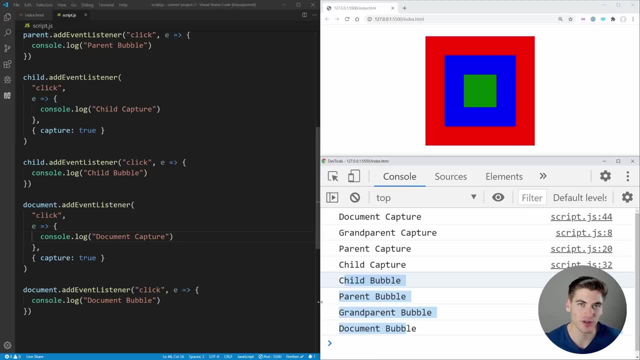 then goes from the inside and bubbles outward. That's how these events work. Now, this is all great that we have the capture and bubble phase, but sometimes there are things that are going to happen that prevent the event from going through the entire capture and bubble. 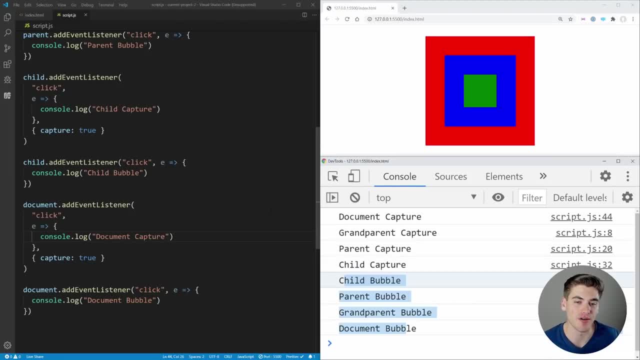 phases And this is what happens when you stop the propagation of an event. So let's say that when we get to the parent capture, we want to stop all propagation. We want to say you know what, once the parent gets the event, we want to stop and have nothing else. 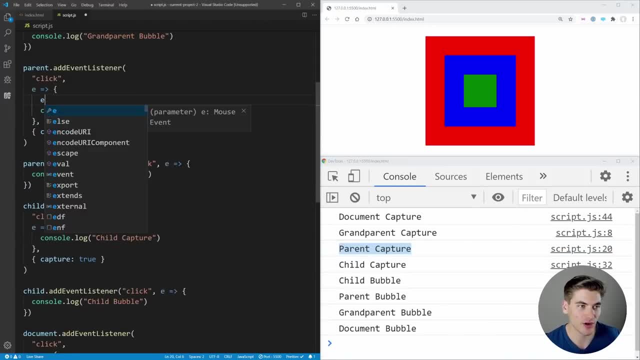 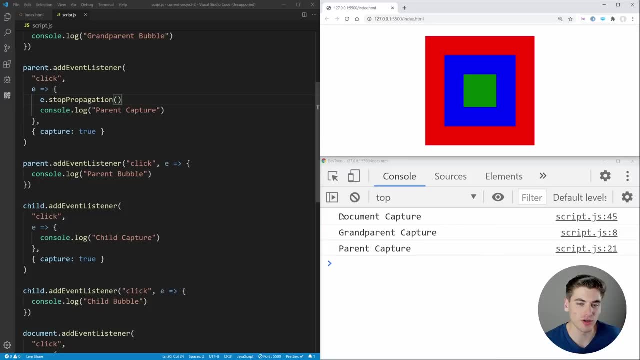 get it. So if we find our parent capture here, we can take our event object, which we call e, and call the stop propagation method on it. Now when we click on the child, you're going to notice it goes: document capture, grandparent capture and parent capture, and then none of the other. 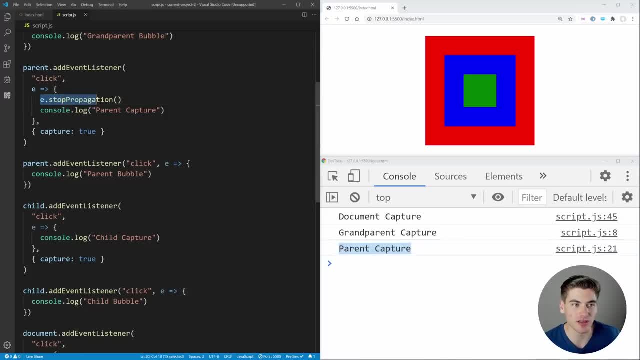 capture phases or bubble phases occur Because what we did here is we stopped the propagation of our event, which means it just immediately stops. It doesn't do any more capturing or any more bubbling, which is why we only get these three being printed out. 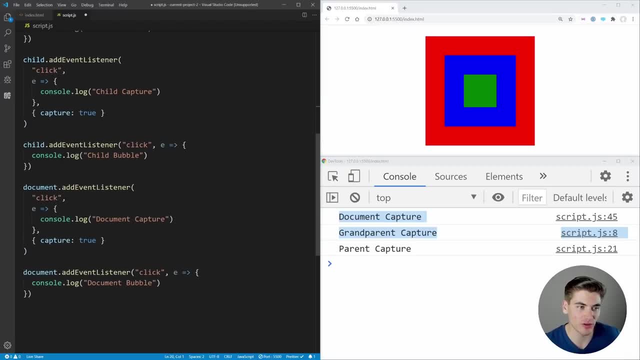 If we move this now instead into, let's say, our child bubble and we just paste it in here, you're going to notice it goes through the whole capture phase for all of our elements And then, as soon as the child bubble happens, it stops propagation and none of the other bubbling for. 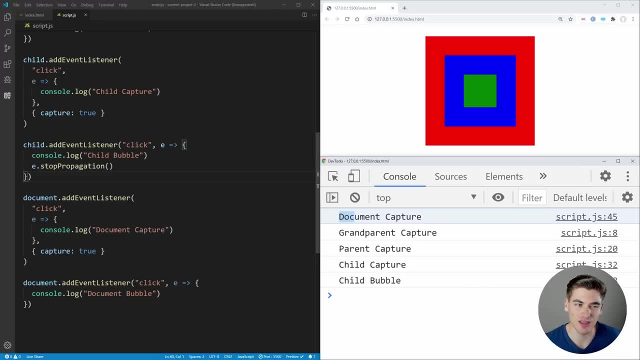 the parent, grandparent or document occur, So we can use estop propagation to stop our event from propagating upwards Or downwards through the capture or bubble phase. Now I just want to clean this up a little bit. We're going to get rid of our document events and we're going to get rid of all these capture. 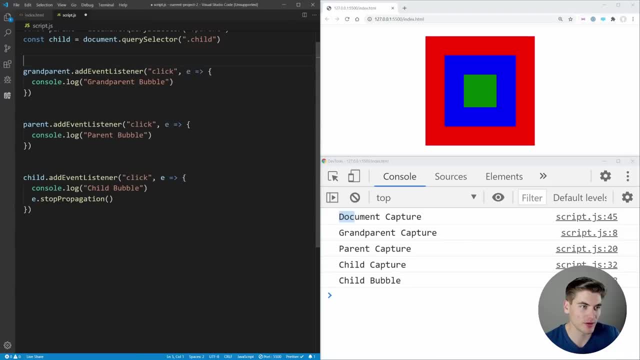 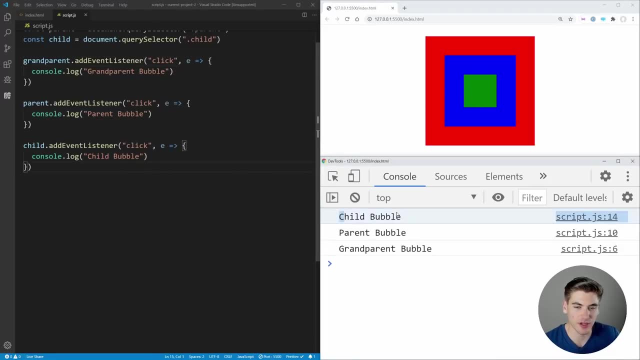 events as well. So we're just left with our original three events that we set up here. So we have grandparent, parent and child And when we click, if we get rid of this, stop propagation- you can see we get child bubble, parent bubble and grandparent bubble. 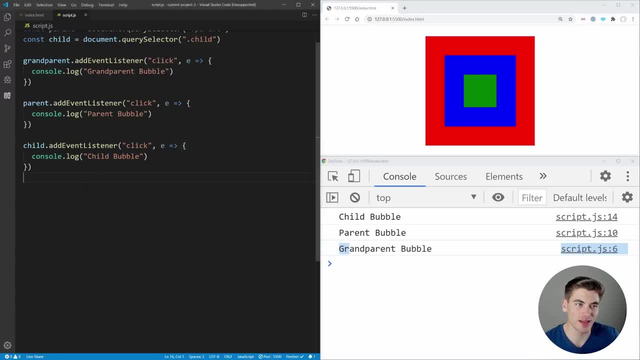 Now, another thing I want to talk about is a really common thing that you need to do with events, and that's when you want to run an event once and never run it again. You can use this third parameter here inside of your add event listener and you can pass it a property of once Set that. 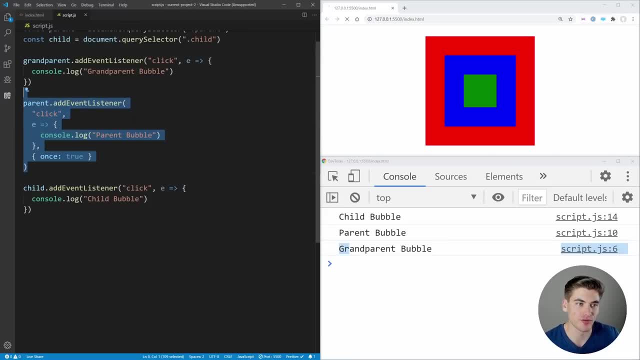 to true, and this event will run one time and then remove itself immediately. So if we click, you can see we got child, parent, grandparent. Click again, we just get child and grandparent because parent was set up to run only one time, which is really useful if you need an event just. 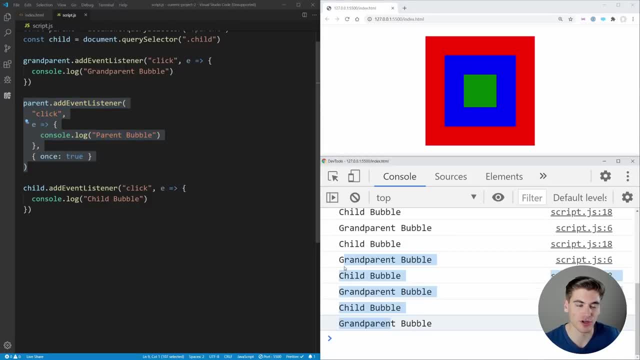 to happen one time And we can click as many times as we want. the parent is never going to show up here. What happens if you maybe want an event to run three times or four times or five times, or you want to stop it on your own? 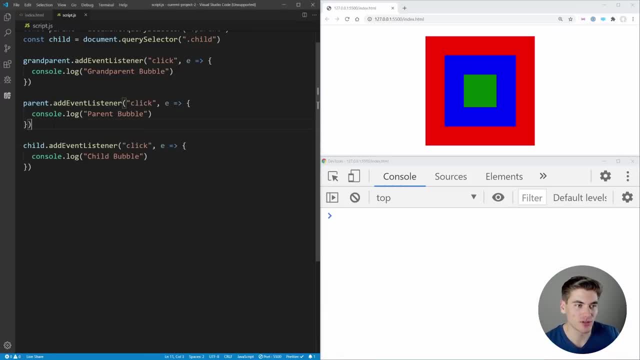 Not just after one event. but what you can do instead is use the dot remove event listener function. This works just like the add event listener: You pass it the type and function and it will remove that function from your event listener. So if we just come down here, 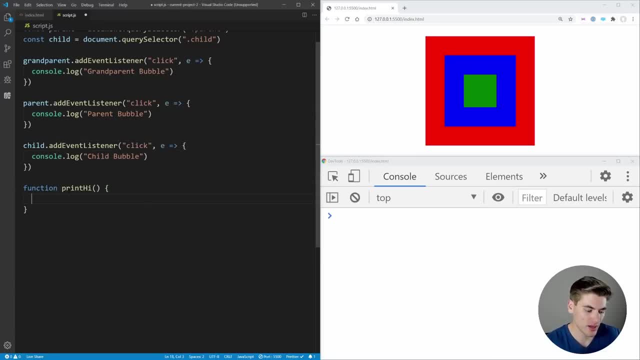 and create a function called print pi and we just say: consolelog pi, make it capitalize. there we go. And when we do the parent here, what we want to do instead is print pi, Then we can remove that event listener at a later point. So let's just say: 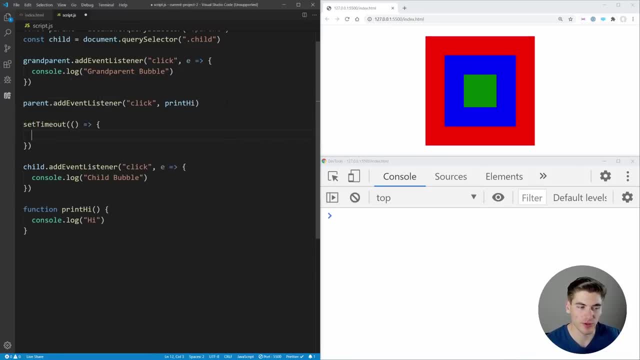 set timeout And this is just going to run some code. after, let's say, two seconds, So 2000 milliseconds, we're going to do parent dot, remove event listener on the click event And we want to remove that print high function. So now if I run this and I click, you can see it prints out high. 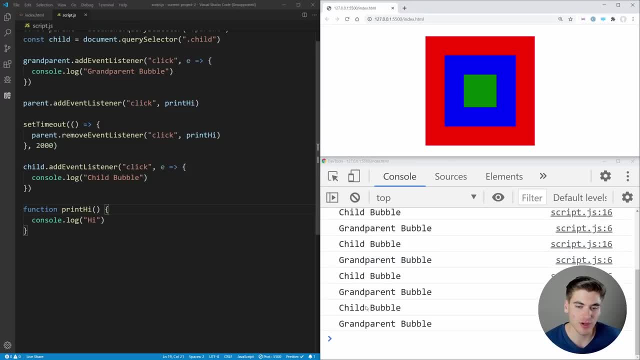 for our parent. But if we wait you know two seconds and then click again, you can see it has removed that event listener. So now if I run this and I click, you can see it prints out high for our parent. And the reason I created a function separately for this is that if we wrote this: 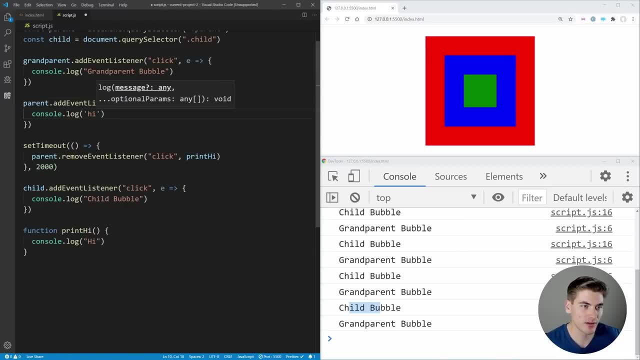 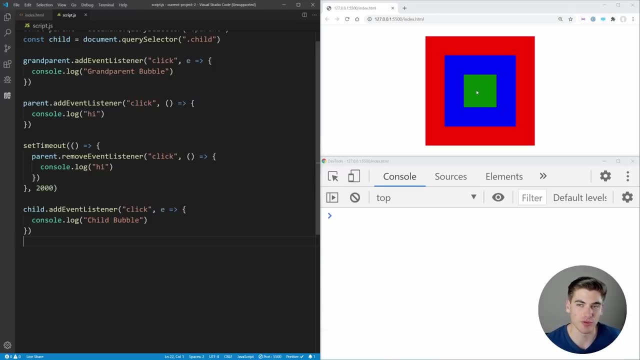 code in line like this consolelog pi and we just copy this over here. remove this function down here. you're gonna notice this doesn't actually work. we can click a bunch of times, prints out high And now if we wait two seconds- it's been about two seconds- we click again, it's still. 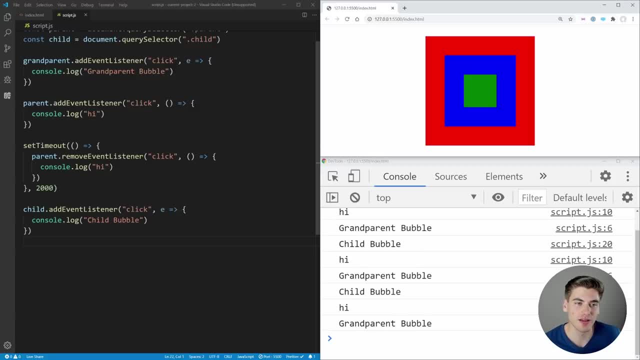 printing out high, as you can see here, And the reason for that is that this function and this function over here, while they look identical, are actually two different functions, because you created two anonymous functions, So they aren't the same, which means remove event. 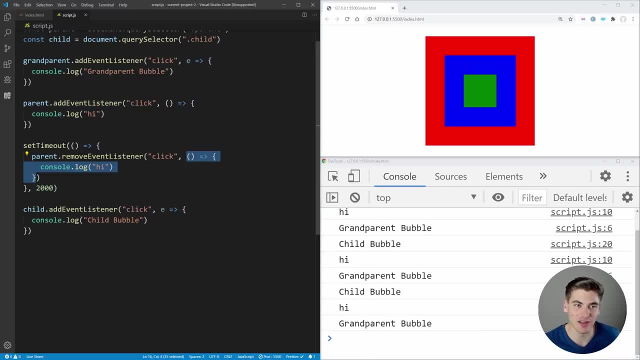 listener can't remove it because this event is technically a new event And it's different from the original event we added it to. That's why, if you want to use remove event listener, you need to create a variable or function or something that is the same for both of the add and remove event. 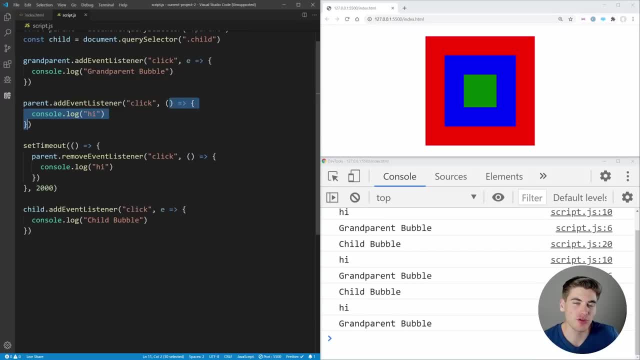 listener. Now, the very last thing that I want to talk about is going to be how you delegate events, really important when it comes to dynamically adding elements to your page. Let's just get rid of all that And we're just going to select all of the divs on our page. So, document dot query. 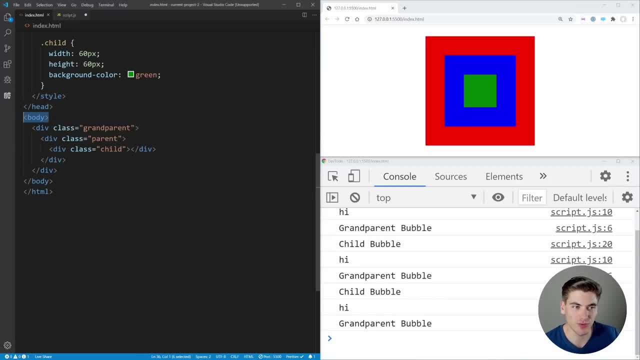 selector all for our divs And each one of these elements is a div. So it's just going to select all of our elements And then we just want to loop through our divs. So we'll say, for each div, all we want to do is add an event listener. Oops, not console log. div dot. add event listener on. 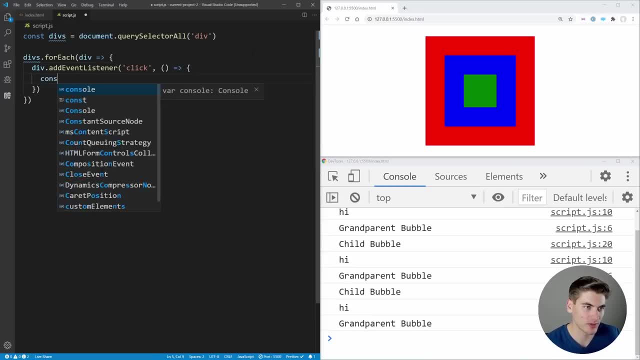 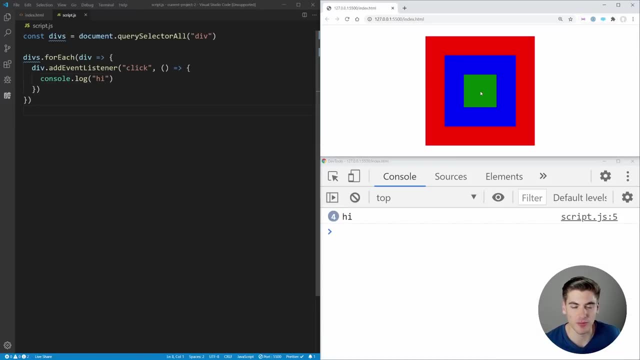 click And we just want to print out, for example, console dot log. Hi, there we go. Now, when we click on a div, it's going to print out high. if we click on one of the middle divs is going to print high for each one of them. That works just. 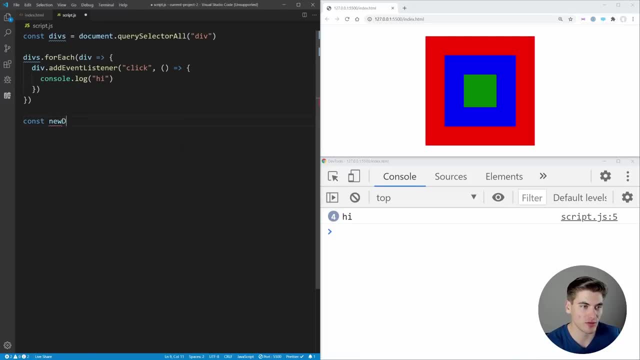 fine. But now let's say that we want to create a new div. So we're gonna say: new div is equal to document dot, create element of div. And then we're just going to append that to the end of our body. So body dot, append new div. Let's make sure we just give this div some style so we can see it. 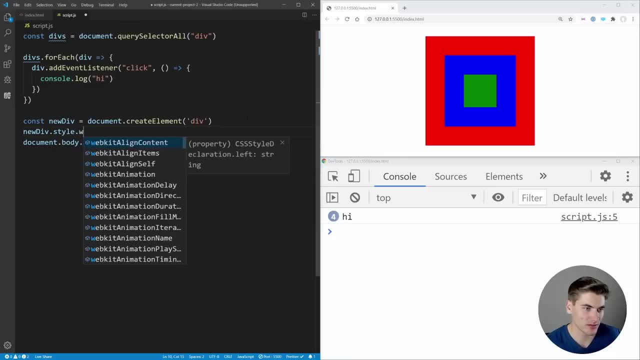 The new div dot style Dot width equals 200 pixels. New div dot style dot height equals 200 pixels And we'll just say new div dot background. I'm sorry, dot style Dot background color. we're just going to set this to purple, So now you can see we have this. 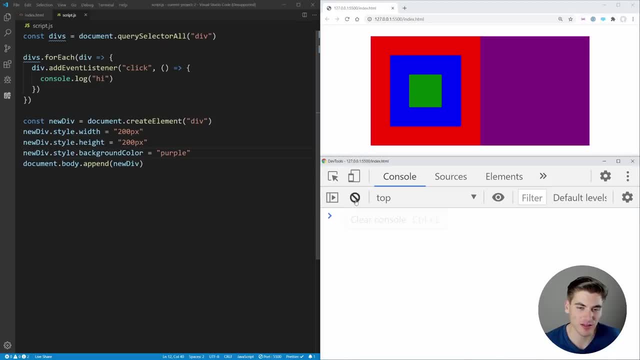 new div over here And when we click these divs they all print out high, just like we expect. But when I click this div, it doesn't print high, And the reason for that is that up here I selected all of the divs on my page, I added event listeners to them And then, after I did, 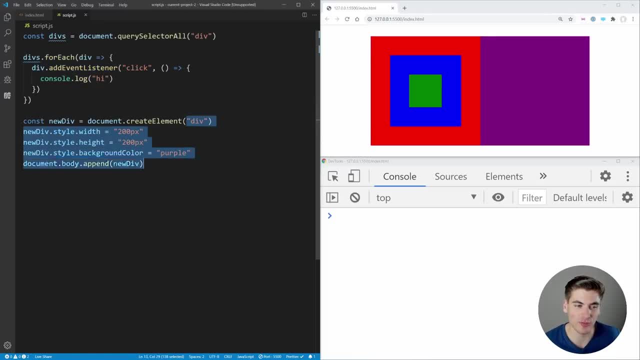 that I added a new div And then I, you know, put it on the page, But this one wasn't selected up here because the selector was ran before I created this new div. This is a problem a lot of people that are new to JavaScript and event listeners run into. is they think that the new div will have the 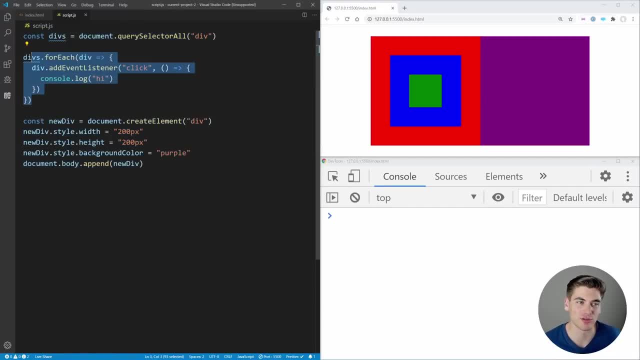 event listener. but it actually doesn't, because it was added. after the event listeners were added, We could come in here and say new div dot, add event listener or click, And you know we could come in and make sure that we console log high inside of here. And now it'll work because we added the event listener after. 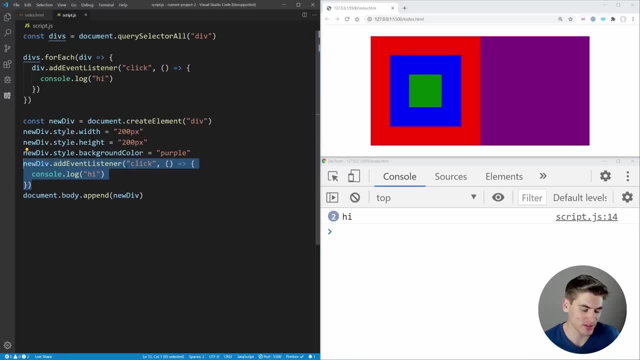 the fact this is kind of clunky and it's really a pain to do this. So instead, what I like to do is event delegation, Since you know that our events go through the bubble and capture phase. we know that all of our events eventually end up on the document. 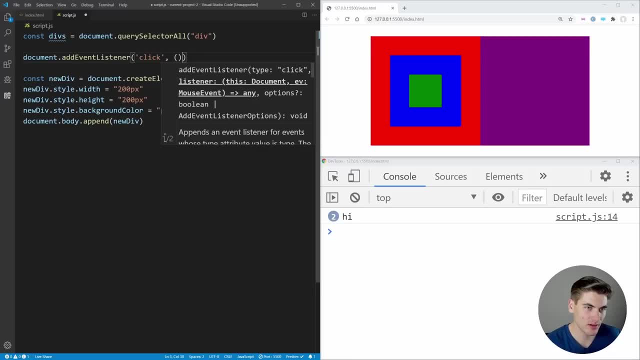 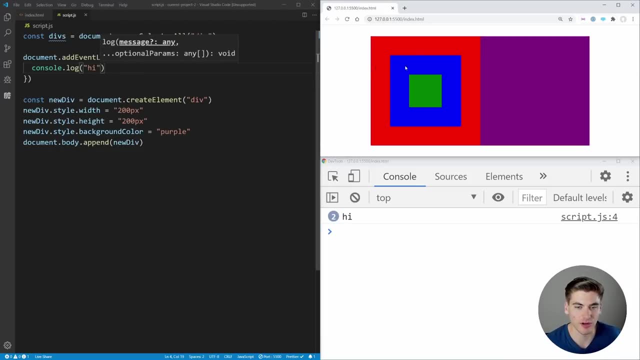 we can say document dot. add event listener for click And then see inside of here we can just console dot, log Hi. Now what this is going to do is just log high every time we click on our page, whether we click on one of our divs or if we click on our body or anywhere else. So 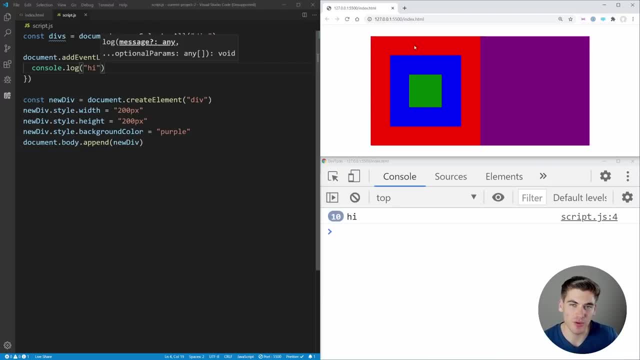 clearly it's not quite what we want, because it works everywhere And we only want it to work when we click on a div. So what we can do is take that event property called E, we can get the target from it And we can call a function called matches. This just takes a CSS selector And if 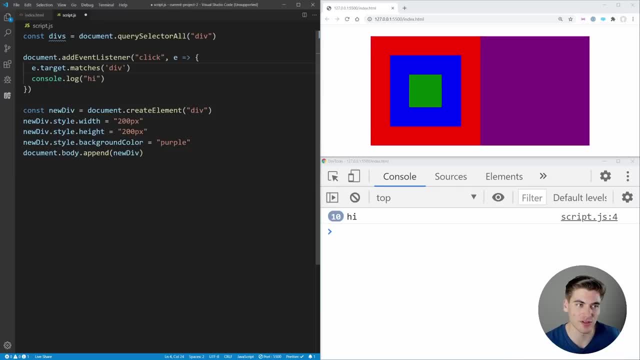 the target matches it, it returns true, So we could pass a div as our selector here And then, if this is true, that means we've clicked on a div, So let's log out high. And now when I click inside of a div, you can see we get our high being logged out, But when I click over, 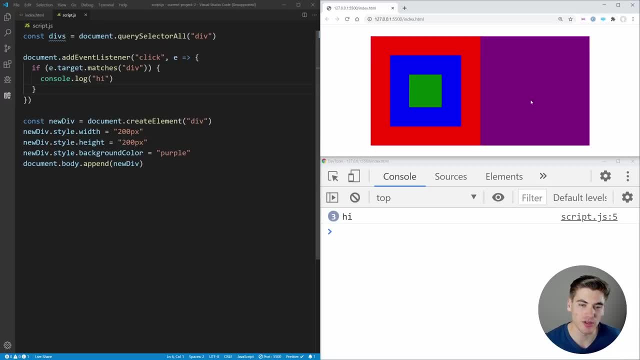 outside of a div, you notice no highs being printed, But our new div will print out high, just like we want it to. So this is perfect and does exactly what we want. I use this kind of code all the time, which is why, generally, I like to turn this into a function. 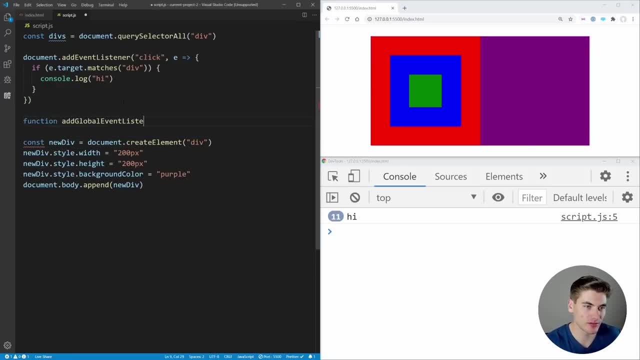 I like to just call it: add global event listener, which takes a type, a selector and then a callback And inside of here I just like to add my event listener. Oops, add the event listener or the type. I like to then have my callback here. 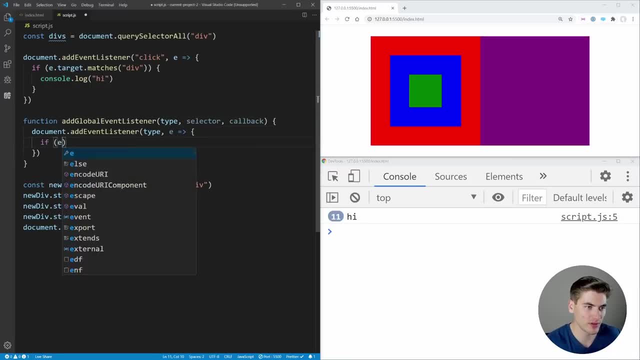 And inside of this what I do is I just say, if E dot, target dot matches- oops, matches selector, then I call the callback with the event. this right here does the exact same thing as what we have up here. So I could just say: 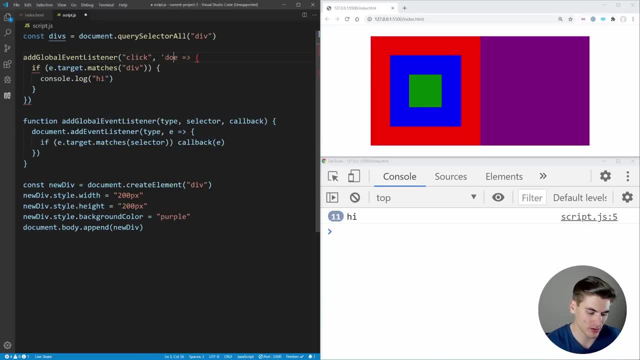 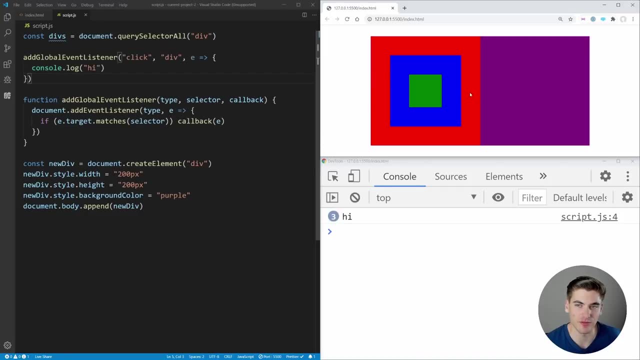 add global event listener for click and I want it to match a div. Then I can just get rid of all this code. And now, if I run this, we get the exact same thing. When we click a div it prints out high and anywhere else it doesn't. 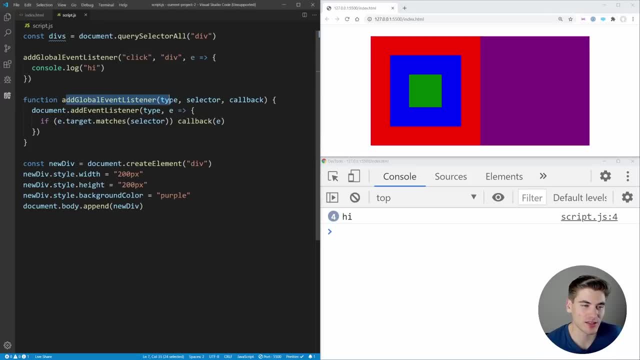 And essentially all that I did is I just wrapped that code inside of a nice handy function which I can call anywhere which takes a selector- I'm sorry, a type a selector- and then a callback for whenever we click on something that matches this selector. 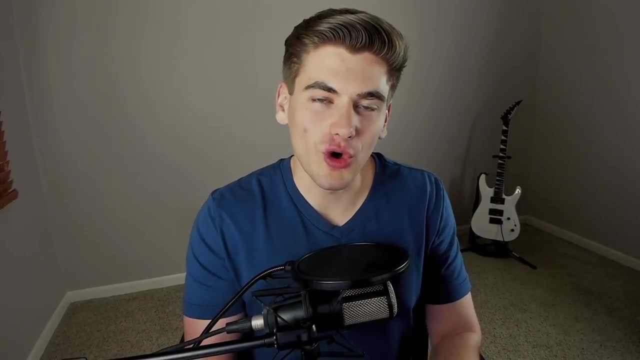 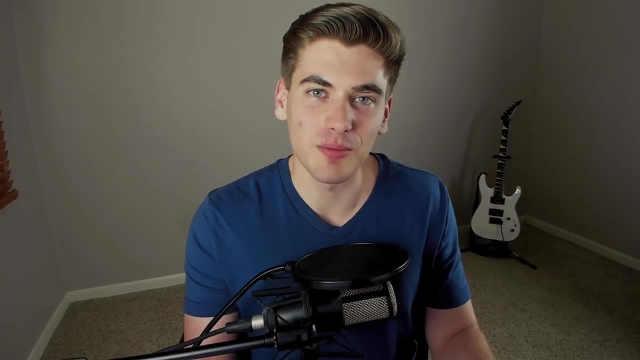 Super handy function. I like to include it everywhere And that's all there is to event listeners in JavaScript. If you enjoyed this video, make sure to check out my complete JavaScript simplified course linked down below. It covers literally everything you need to know. 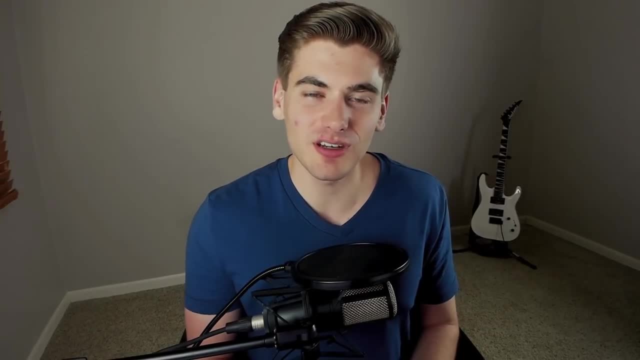 about JavaScript. And, with that said, thank you very much for watching and have a good day.